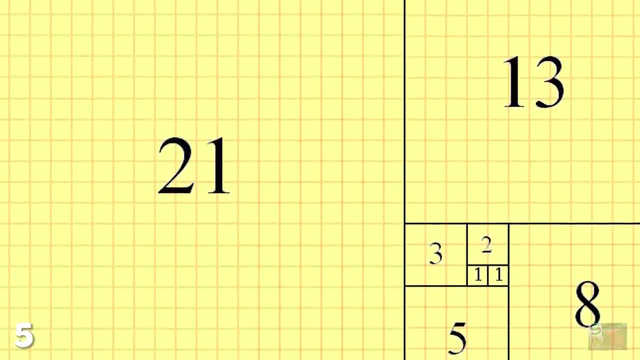 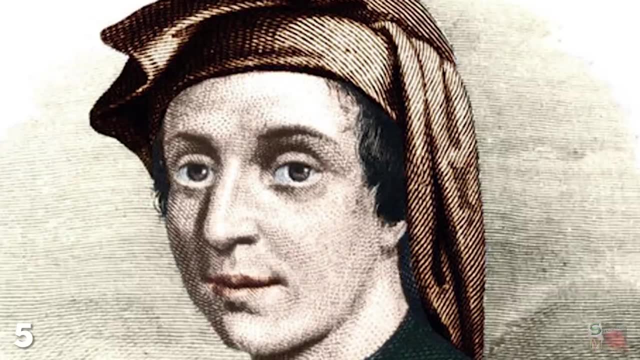 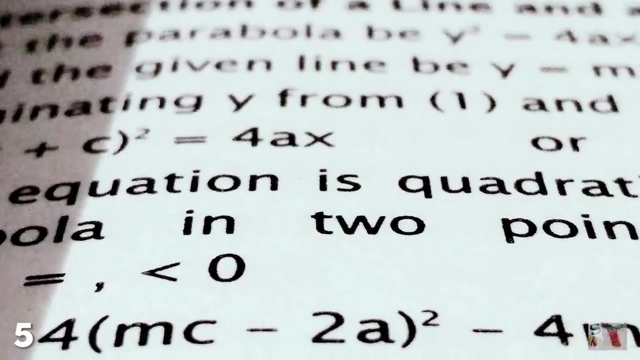 although it had already been identified by Indian mathematicians over a thousand years beforehand. But this guy from Pisa shouted first, so he gets to name it after himself. That's just how things work. As the world began to develop its understanding of mathematics, we soon realized this string of digits was a fundamental 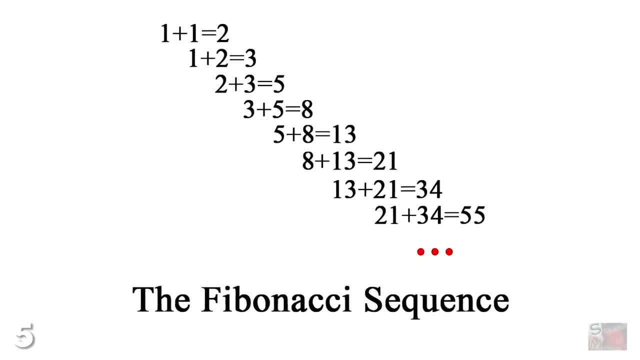 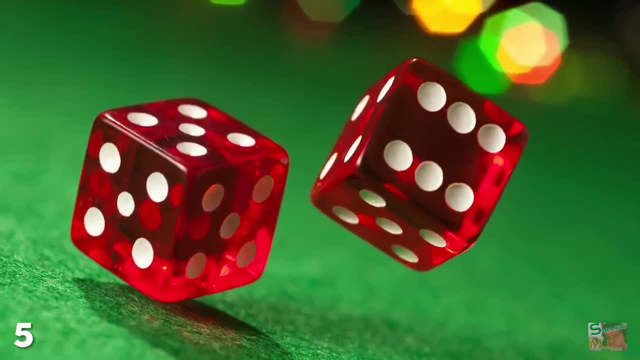 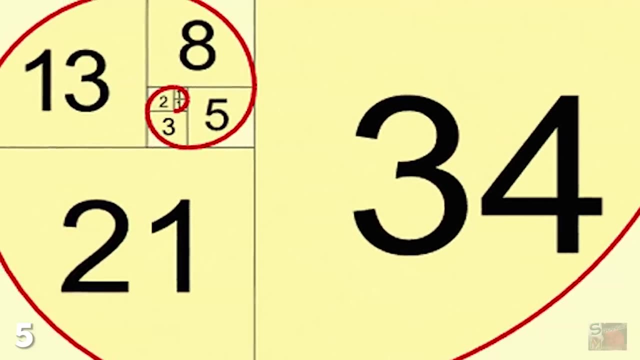 importance, and today we apply this knowledge in all manner of practical ways. Search algorithms, stock trading, gambling odds: all make use of the Fibonacci sequence, But the way in which you have most likely encountered it is via the mysterious golden ratio which appears in. 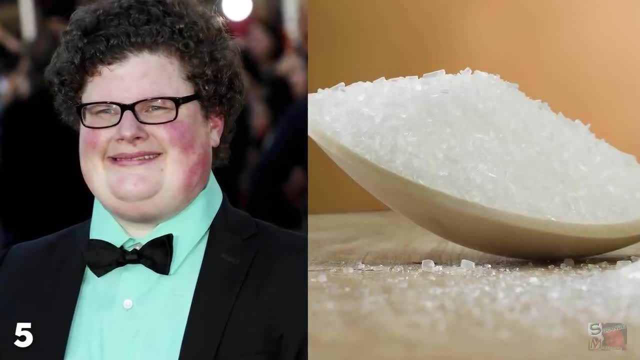 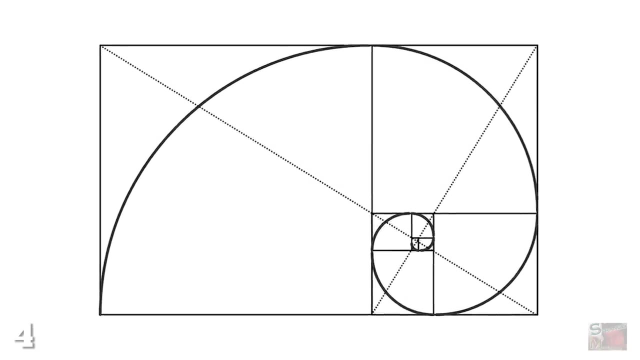 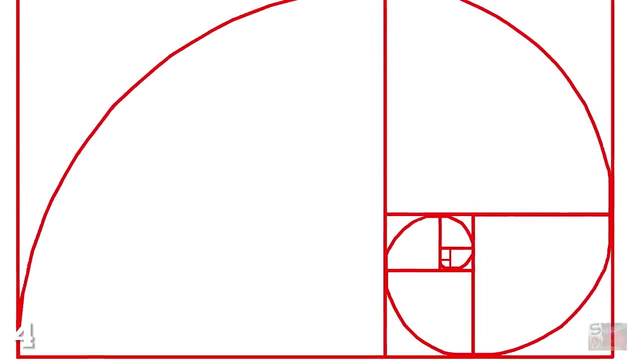 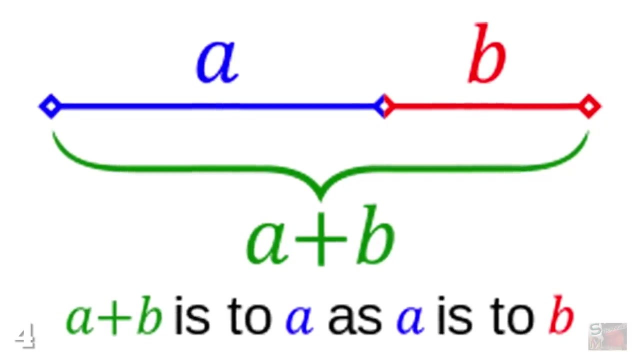 more random stuff than MSG and Jesse Hyman combined Number 4. The Golden Ratio: The golden ratio is a mathematical term used to describe the relationship of two figures whereby the numbers seem to be in some form of complementary ratio. If you have a number A and a lower number B, then the two are in the golden ratio. if the ratio 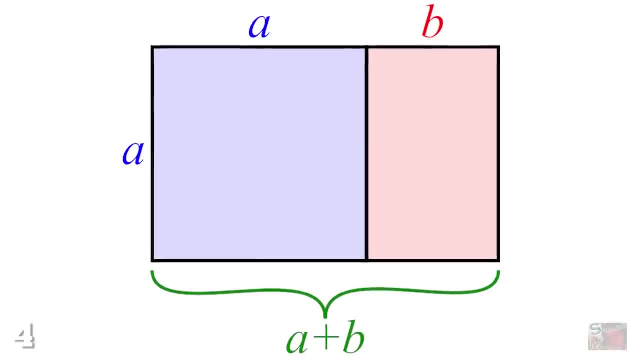 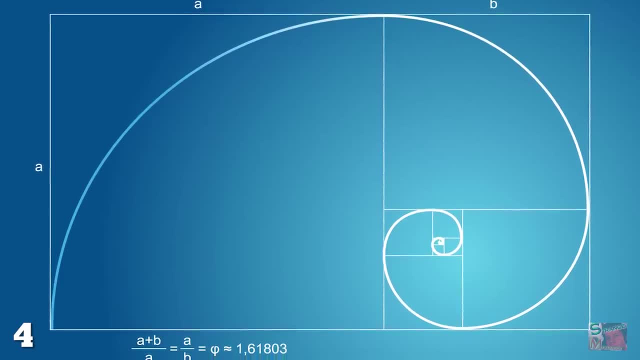 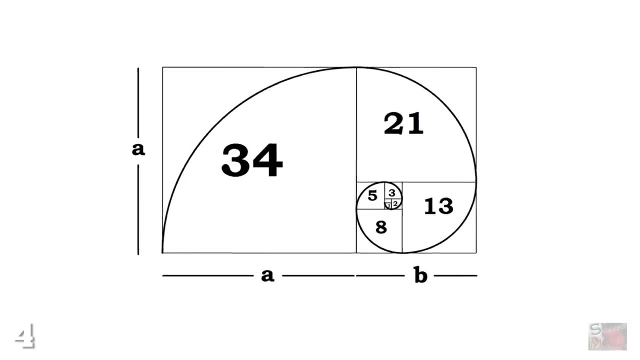 between A versus B is similar to the ratio between the sum of A plus B versus A- A. The Greek letter ascribed to this ratio is phi, and its value is contracted to 1.618034.. Basically, anything which comes close to this value in terms of its ratio is said to be. 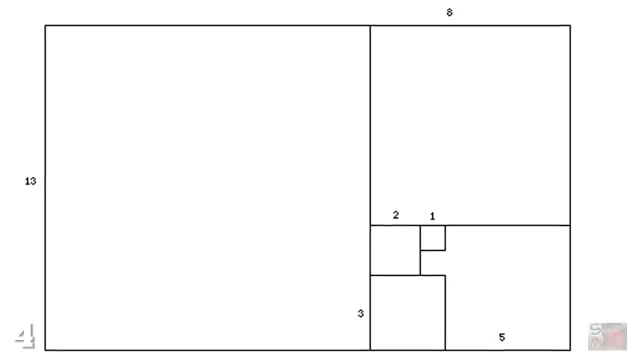 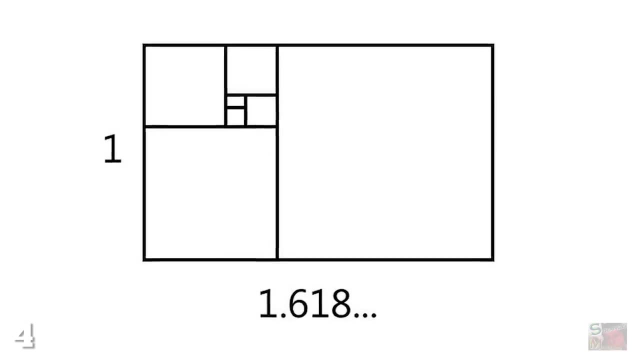 perfectly proportioned. For example, a rectangle that measures 12.94 by 8 centimeters is in the golden ratio, because 12.94 divided by 8 is 1.6175.. And if we add the width and length of, 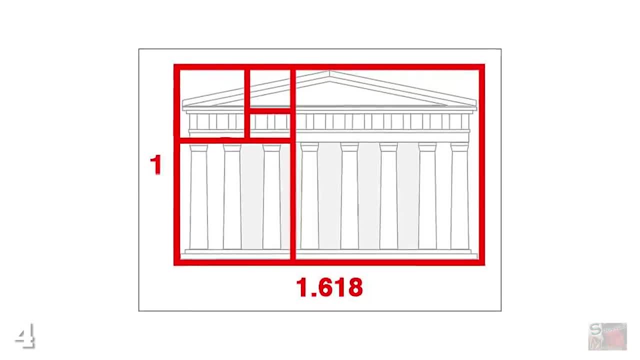 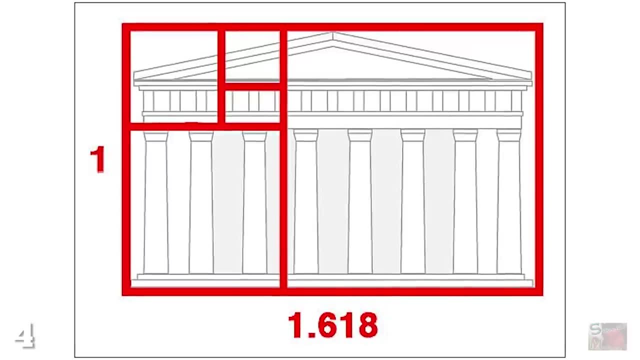 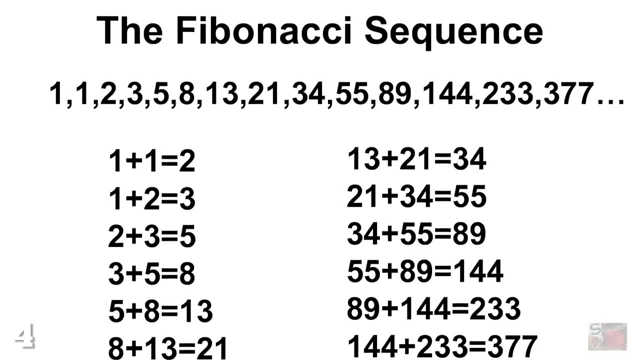 the rectangle together to get 20.94,. the ratio between this and the longer side- 12.94,, is 1.6182.. The golden ratio can be used to calculate perfect spirals, golden triangles and other shapes and patterns too. But what does this have to do with the Fibonacci sequence? 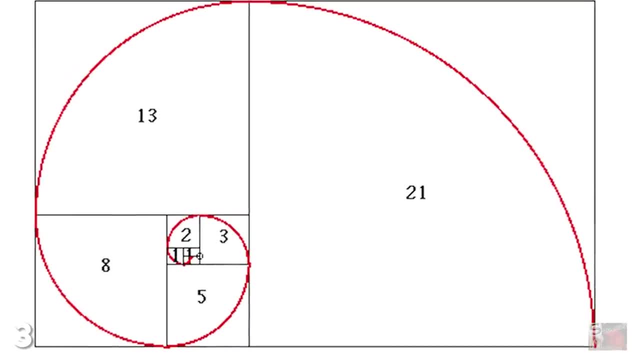 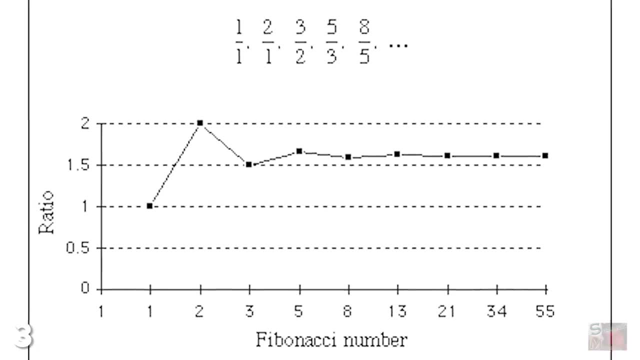 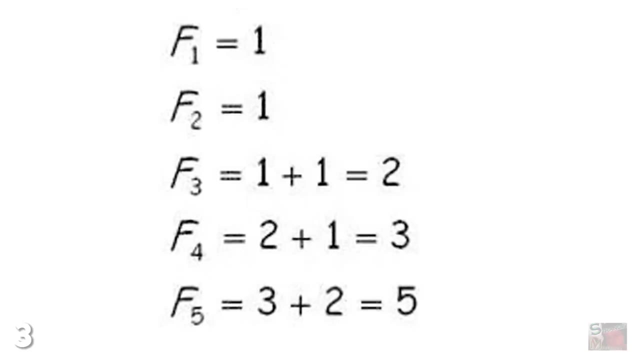 3. The Link To link the Fibonacci sequence and the golden ratio. we must look at the ratio between two consecutive Fibonacci numbers and observe the pattern this ratio takes as you go on, Because it turns out that the further along the Fibonacci sequence you go. 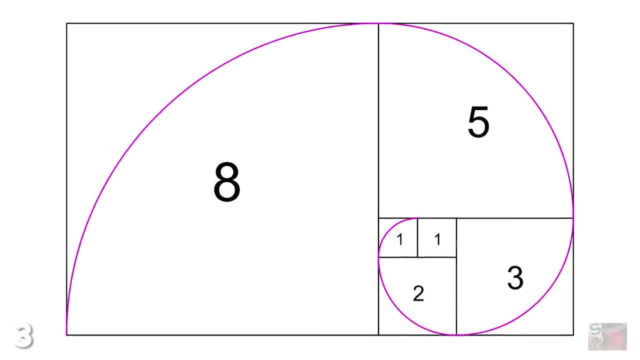 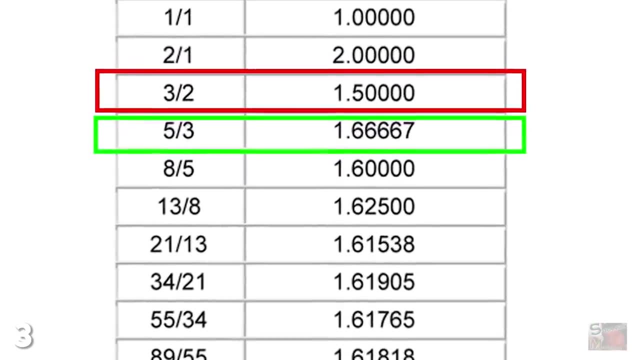 the closer the ratio between any two numbers is to the golden ratio. The ratio between 3 and 2 is 1.5.. The ratio between 5 and 2 is 1.5.. The ratio between 5 and 2 is 1.5.. 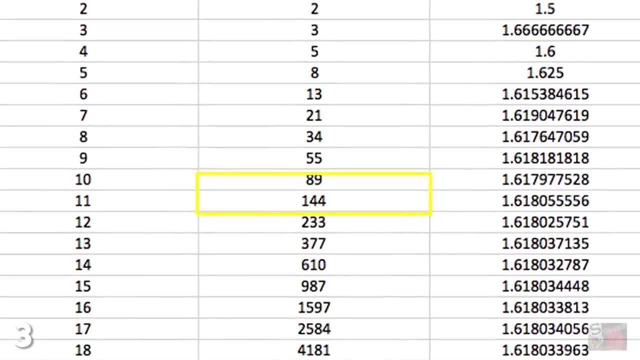 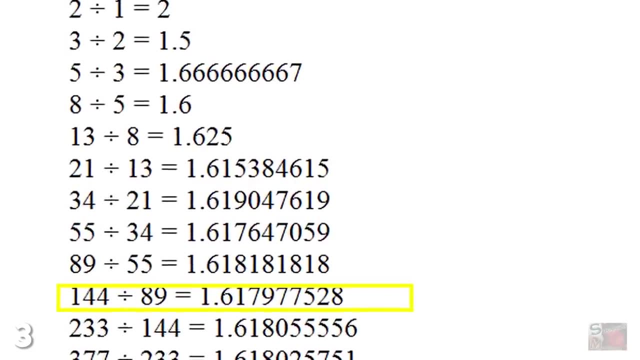 The ratio between 3 is 1.66.. And if we skip along a few to see the ratio between the 12th and 13th Fibonacci numbers, we'll see that their ratio is 1.6179.. The ratio between 144 and 233 is 1.6180,. 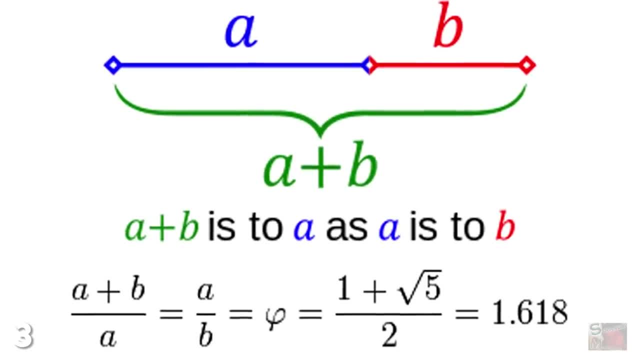 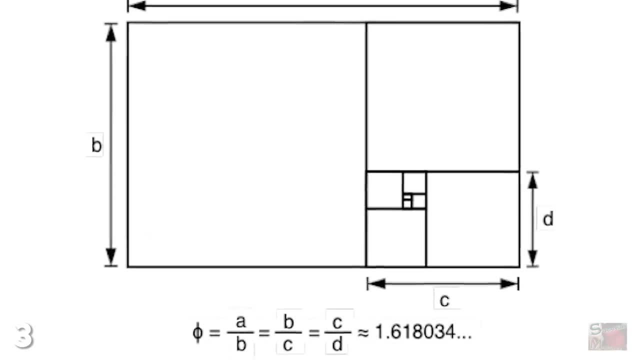 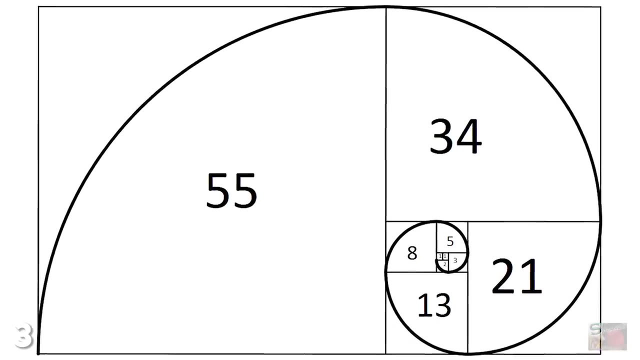 and so on and so forth. As we mentioned earlier, the golden ratio is 1.618034.. So clearly, the golden ratio and the Fibonacci sequence have some sort of link which we haven't worked out yet, And that is why so many smart folks have become absolutely obsessed with it. 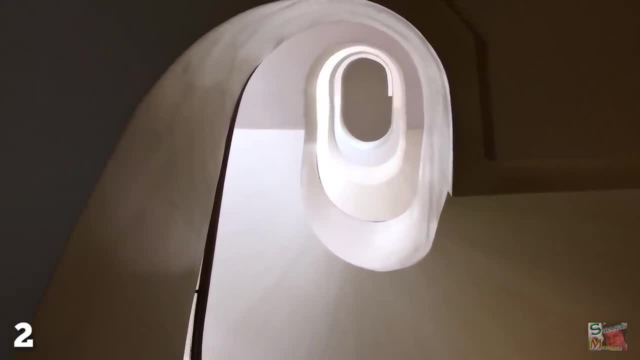 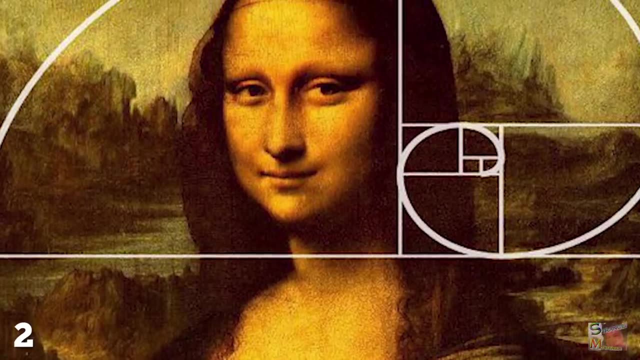 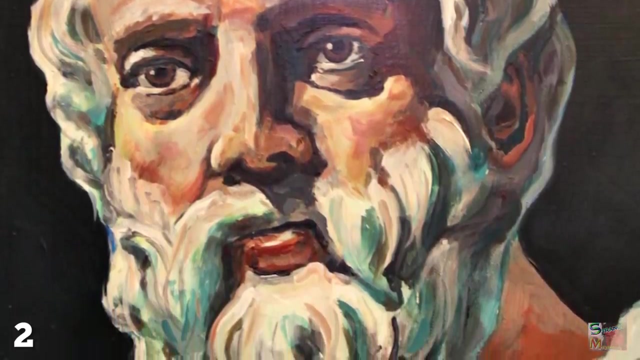 At number two, the uses. The golden ratio has fascinated the world's most knowledgeable people for millennia since its discovery, and we have seen its influence in some of the finest works mankind has ever produced. Plato's study into the golden ratio was used in the designs of the Parthenon. 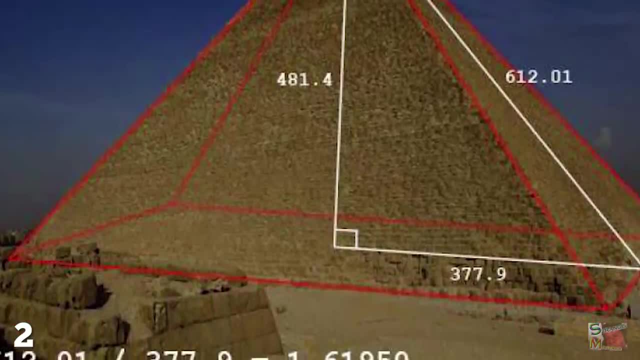 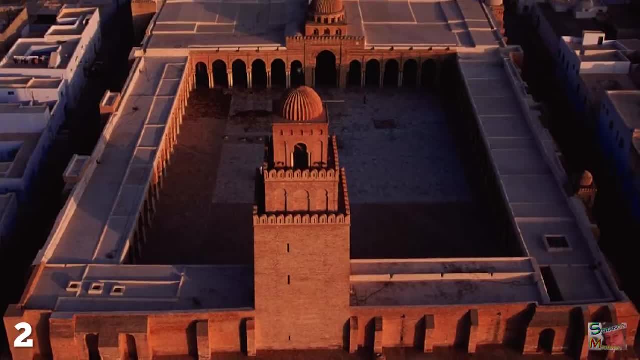 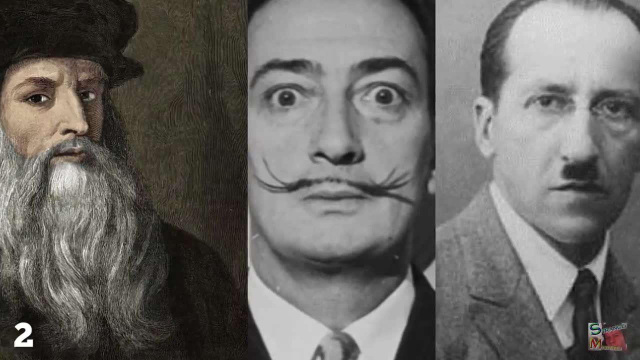 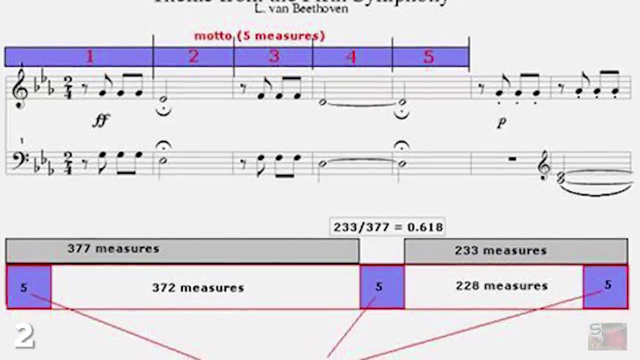 And the likes of the Taj Mahal, Notre Dame and the Great Mosque of Kirhuyan were also built according to this important mathematical law. Artists from Da Vinci to Dali also incorporated the golden ratio in the layout of their paintings, and the ratio can also be detected in the music of Debussy, Bach, Mozart, Chopin and Beethoven. 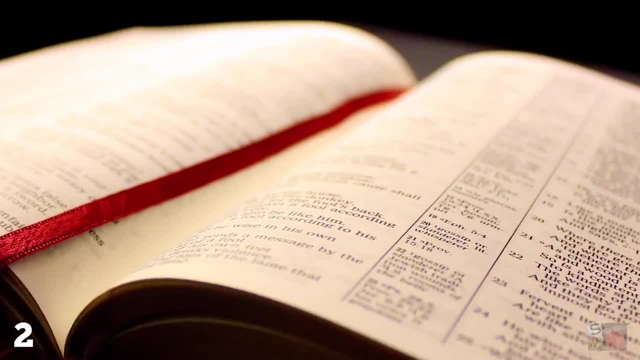 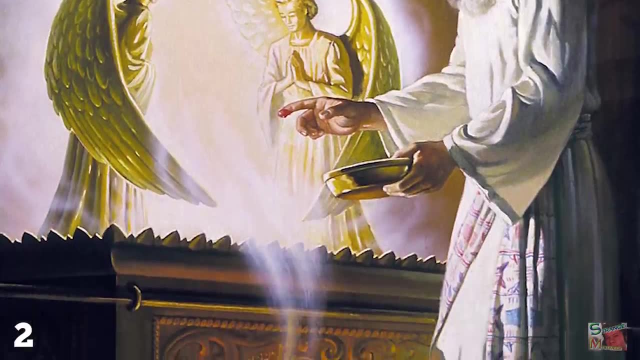 Even the Bible mentions things being constructed in the golden ratio, with Noah's Ark in the, the Ark of the Covenant, both built in accordance with the ratio-driven commandments laid down by God. However, the one thing we're not entirely sure about is whether any or all of this was. 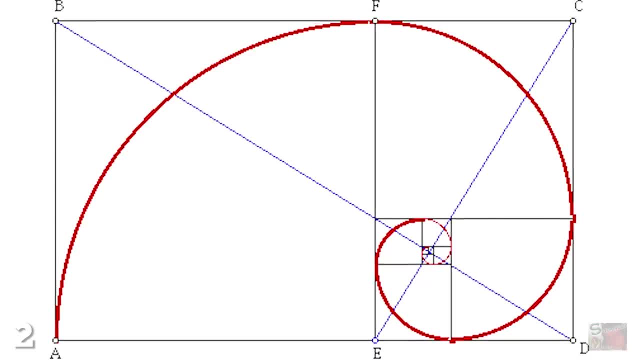 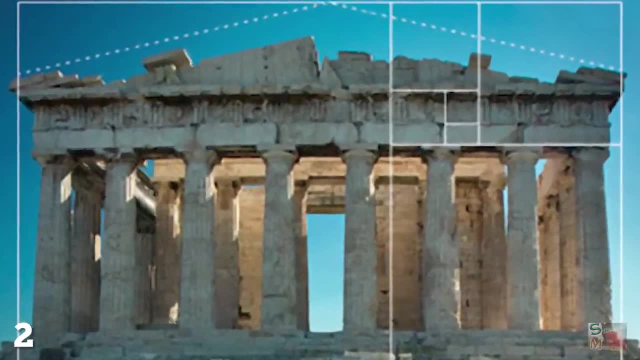 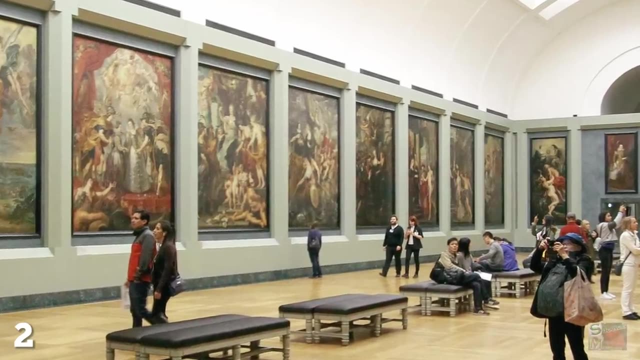 deliberate. Modern artists and architects know about the Golden Ratio and are known to apply it purposefully to their works, and we know that at least some historical buildings and artworks were created by people who knew of the Golden Ratio and its value, But this inexplicably. 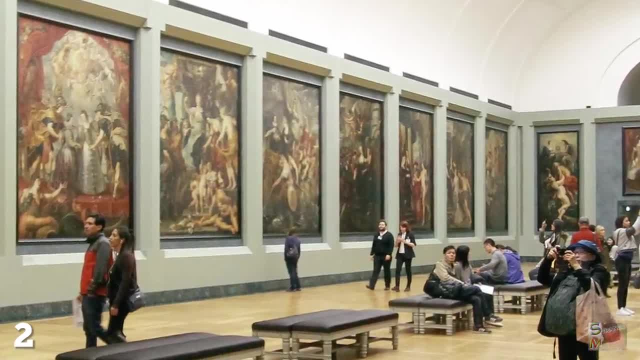 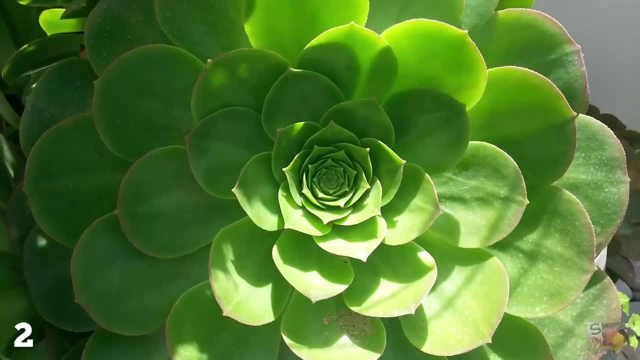 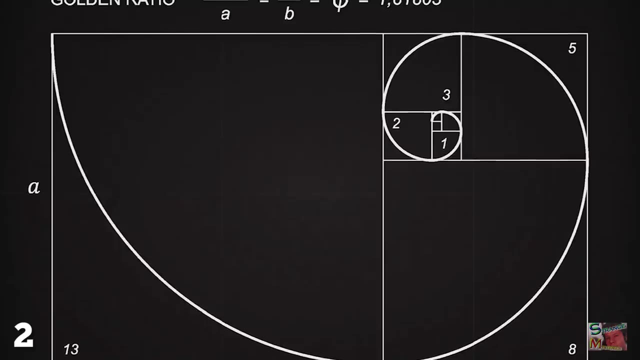 pleasing proportion has been used by people ignorant of its existence too. So is the Golden Ratio merely something which all human beings are attracted to? Is it something that we find inherently satisfying, And is this love of the number 1.618034 limited only to humans? 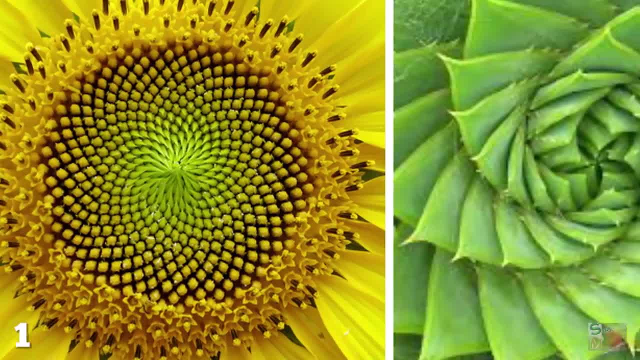 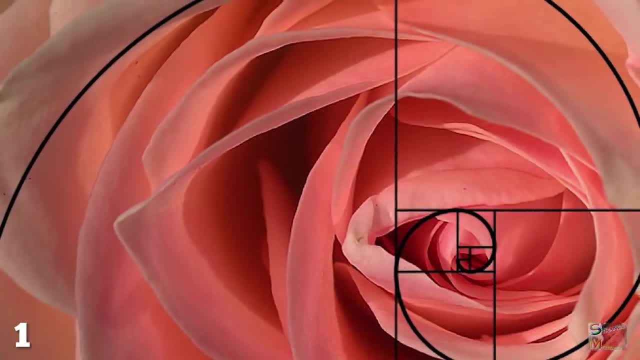 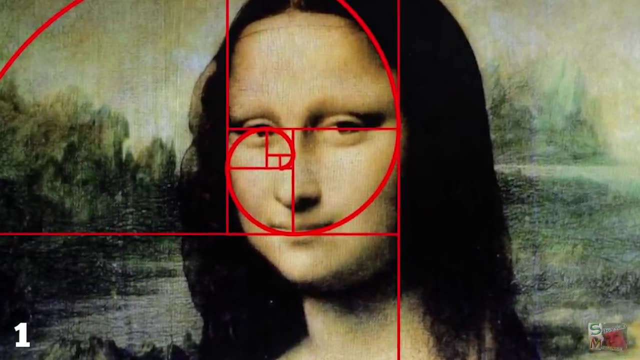 And at number one, nature's design Is the Golden Ratio, a universal law applied by nature. The evidence seems to suggest so, and the aforementioned Leonardo da Vinci may have alluded to this in some of his most famous works. The Divina Proporzioni was a mathematical. 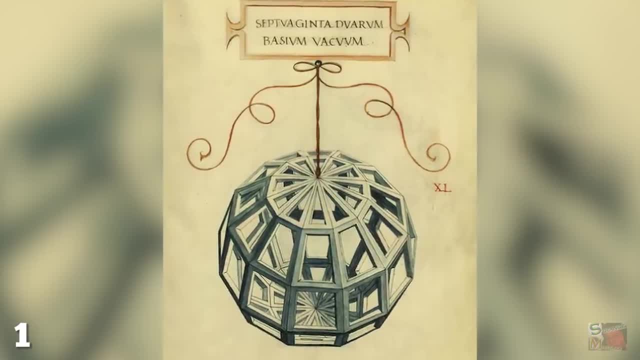 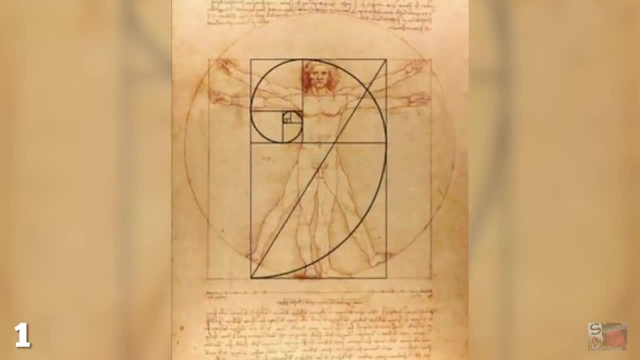 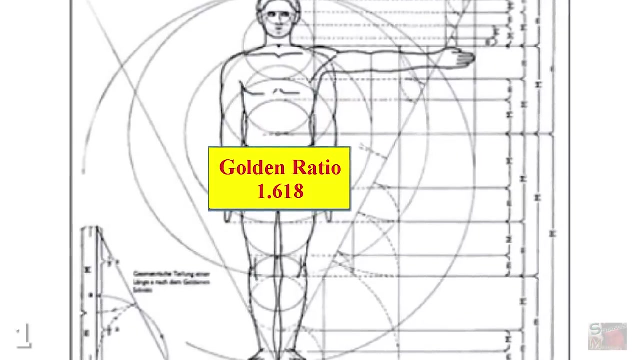 textbook illustrated by da Vinci in 1498,, and in both this and his drawing of the Vitruvian Man he points out examples of the Golden Ratio found within the human body. Psychologists have also found that people whose facial, body and bone structures adhere to the Golden Ratio are often 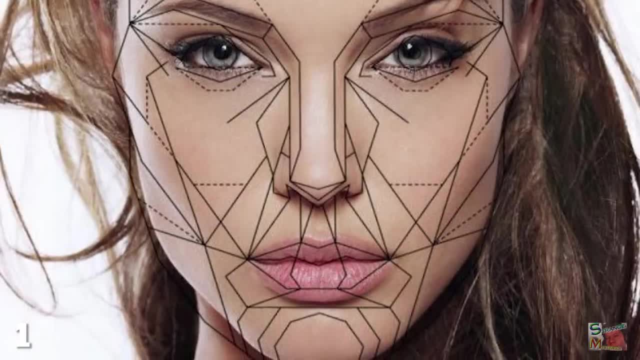 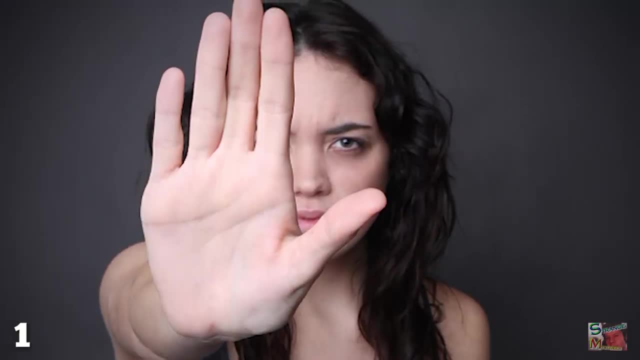 deemed to be more attractive than their non-proportional counterparts. And if you'd like to pause the video to go measure your face right now, we totally understand. But you might want to hold on a second, because the most shocking example of the Golden Ratio within 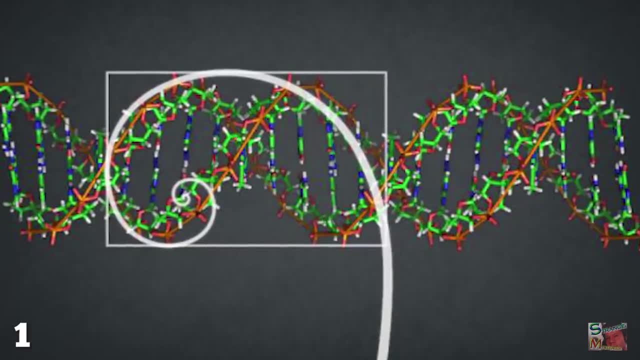 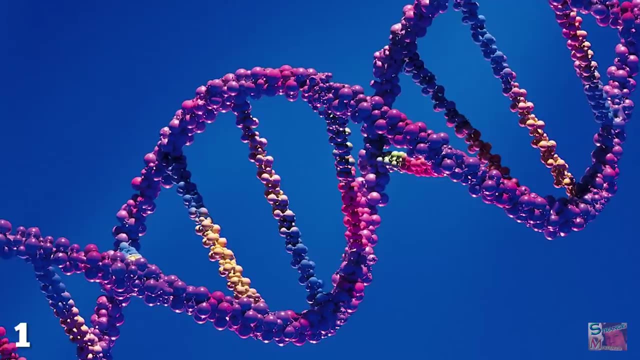 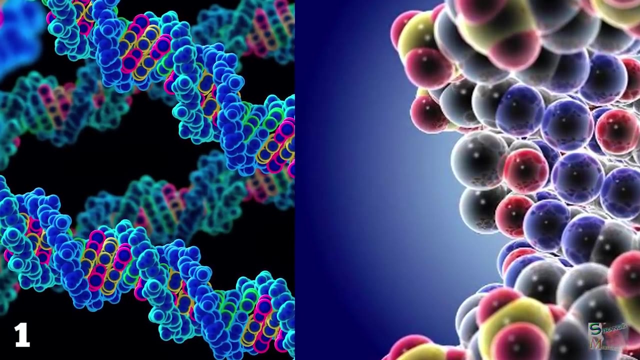 human beings is far more interesting. Did you know that the Golden Ratio even applies to our DNA? The double helix spirals and the composition of a single DNA molecule both seem to have been made in accordance with the divine proportion of the Golden Ratio. And it's not just humans. 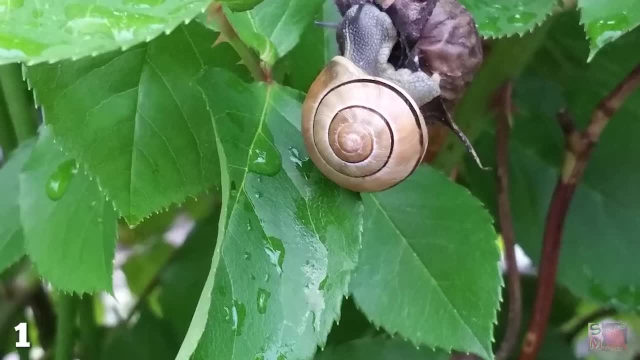 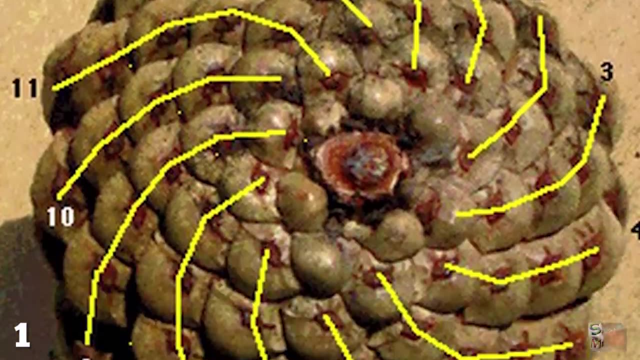 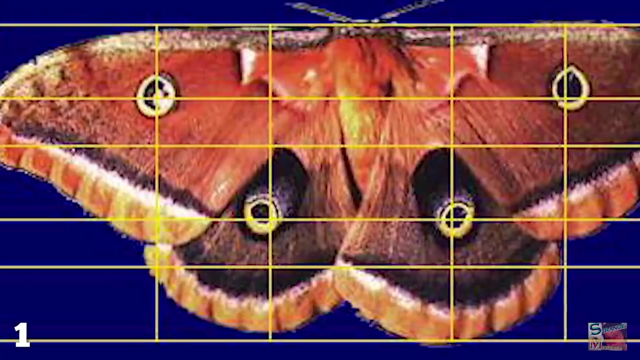 either. as we've seen, the ratio demonstrated in the shells of snails, the number of petals in a flower and the arrangement of individual seeds within seed heads, Pine cones, tree branches and root systems also follow the Golden Ratio, as do some forms of algae and the bodies. 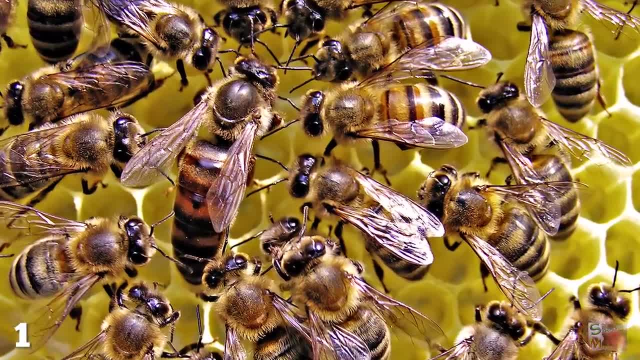 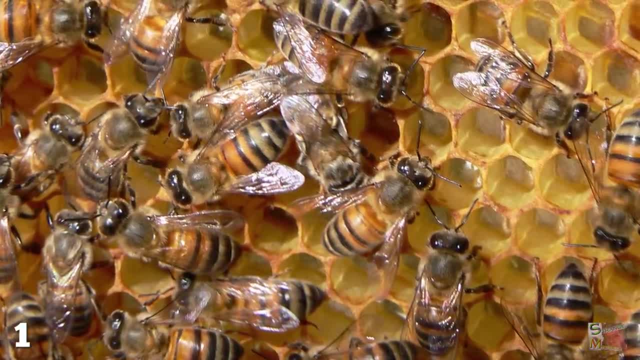 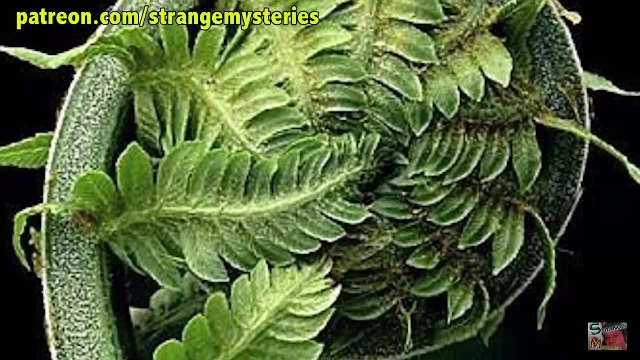 of certain animals. Some creatures even live according to the Golden Ratio, with honeybee colonies known to maintain a ratio of males to females at 1 to 1.618.. So is this ratio evidence that nature has been somehow designed? Was everything on Earth created?